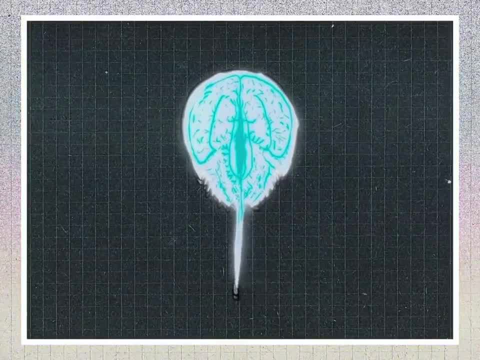 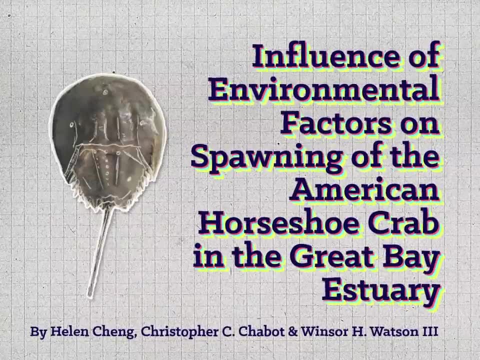 of the water. A 2016 analysis published in the journal Estuaries & Coasts found no clear relationship between spores and crabs. The experiment was to find out the causes of their morning and moon phases, or even high tides. Blasphemy? No. Instead, they observed that the warmer the water, the greater the number of crabs mating and spawning, at least in New Hampshire, where the study took place. They may be like a primordial Goldilocks. 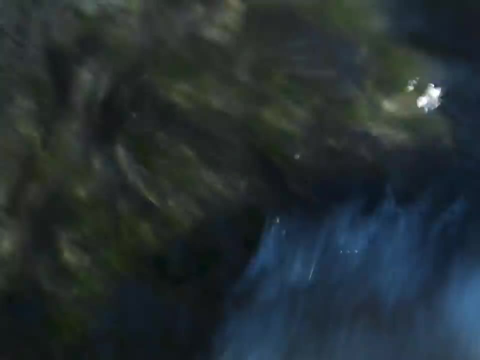 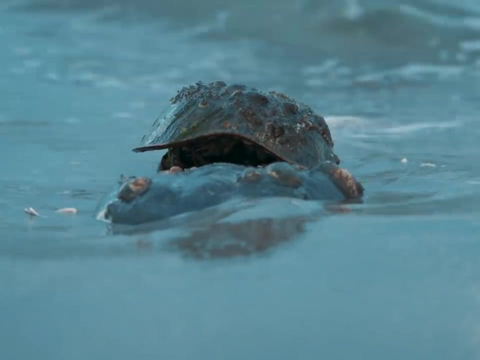 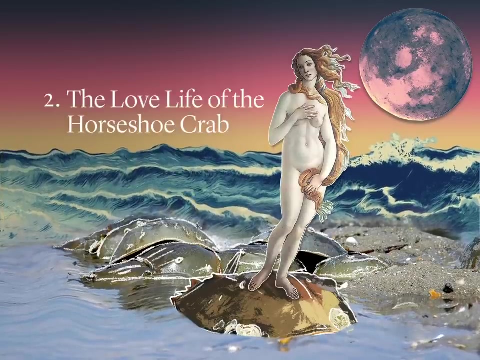 Too hot or too cold and the crabs recede to the depths of the ocean. But when the water is just right, the mating pairs all of a sudden appear. Each spring, horseshoe crabs surface along the coast of the Atlantic Ocean. 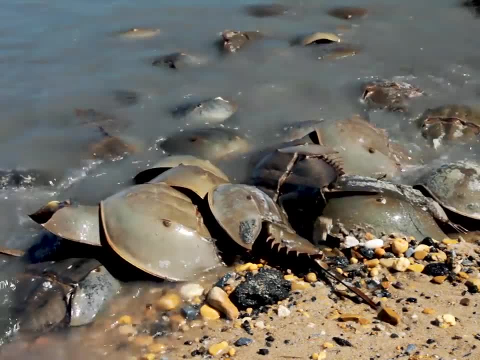 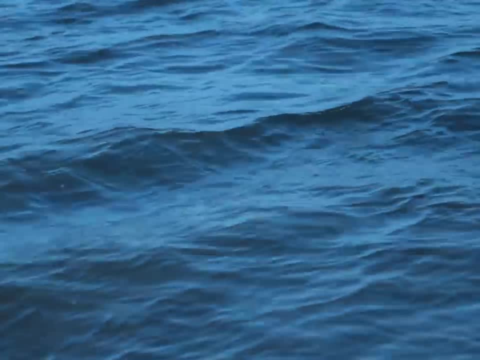 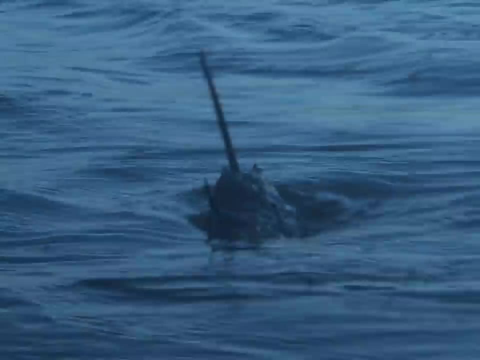 from Maine to Florida and into the Gulf of Mexico or here in Brooklyn, New York. They swim toward the sand upside down, but when they hit the high tide line, they use their telson, a harmless tail, to flip themselves over. 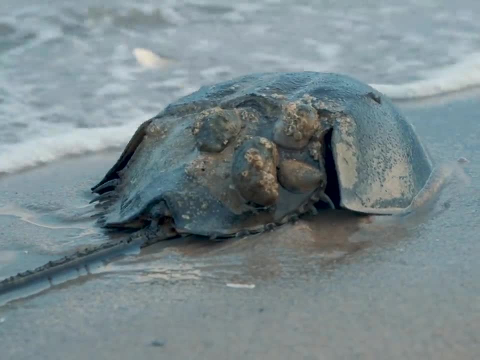 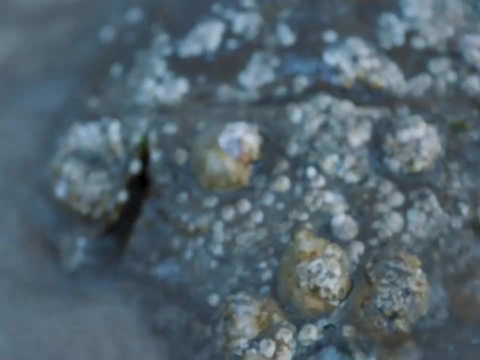 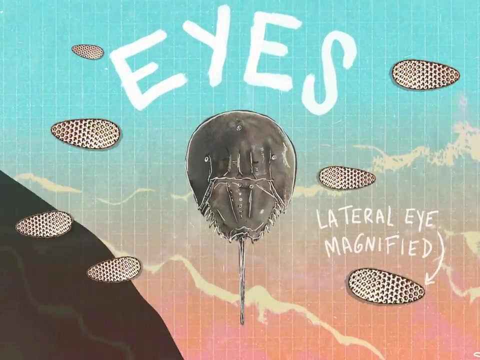 Once righted, they waddle along the sandy ground, carrying other creatures with them: Algae, flatworms, mollusks, barnacles, bryozoans. Their many eyes serve many different purposes. Some see shadows, Others help them identify mates, even in the darkness. 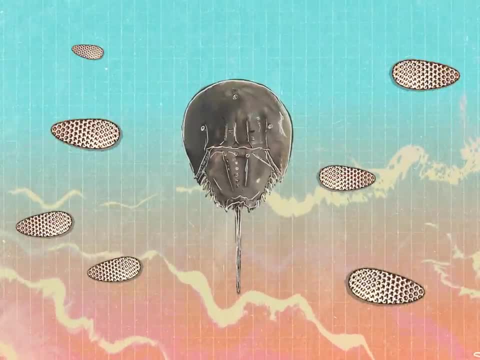 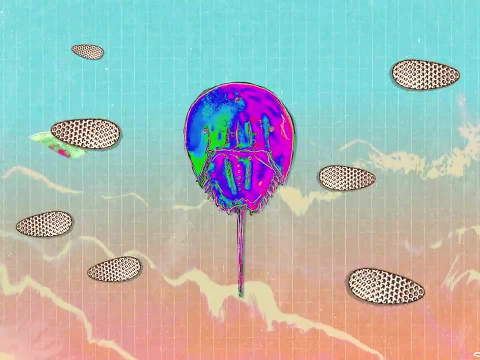 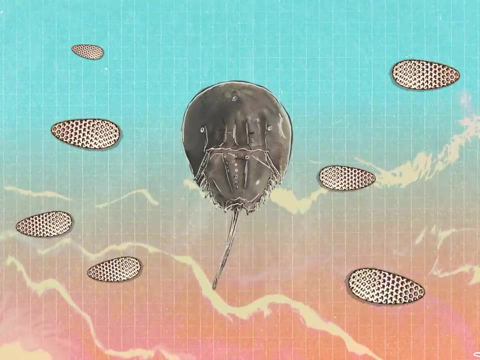 Several eyes are just there to detect UV light, whether it's emanating from the sun or reflected by the moon. They even have photoreceptors in their telson, which lead some scientists to consider the tail an eye of its own, On land and at sea. 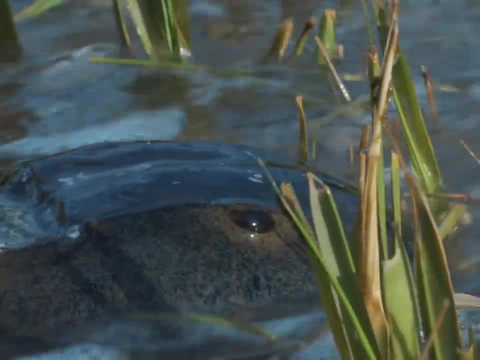 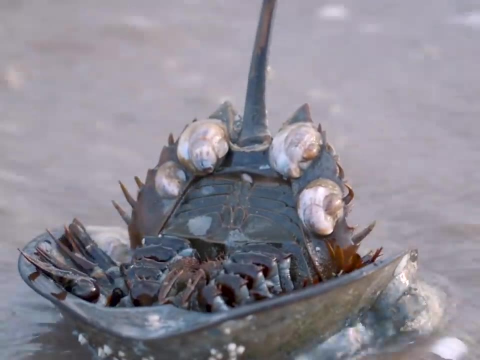 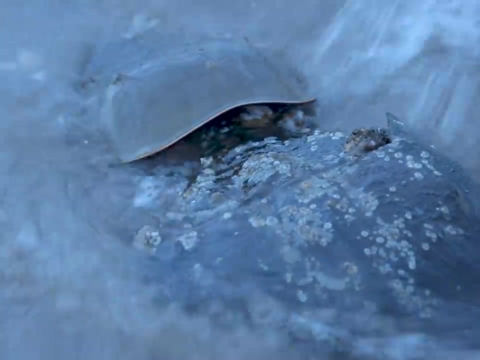 these arthropods breathe with several sets of book gills, each with more than a hundred thin pages. Of course, this book is also a romance. Male horseshoe crabs are smaller than the females, but they use two pincers to attach themselves to the shell of a female. 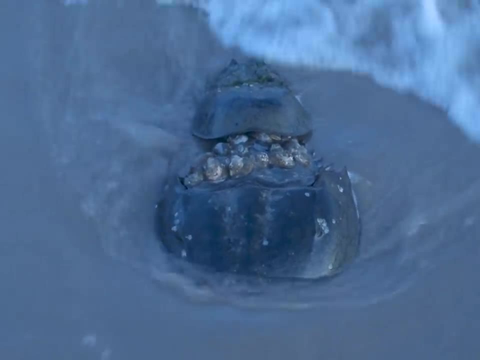 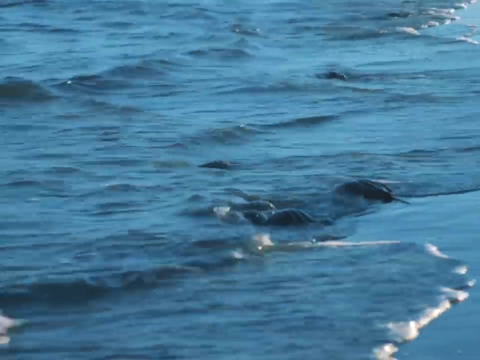 who pulls them up to shore. When she is ready, she will dig a nest and lay a cluster of wet, sand-colored eggs, up to 4,000 at a time. The attached male and any other males orbiting nearby hurry to fertilize them.